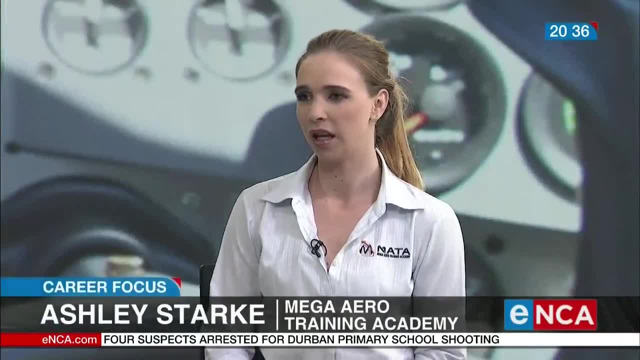 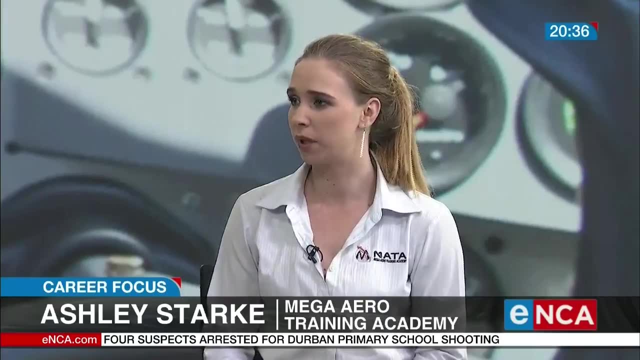 So in avionics, you need to know that there are different trades involved in this. There's an avionician which is made up of three trades. You get an electronic instrumentation and then your radio radar engineer. So what that entails is that's the guy that's working in the cockpit. 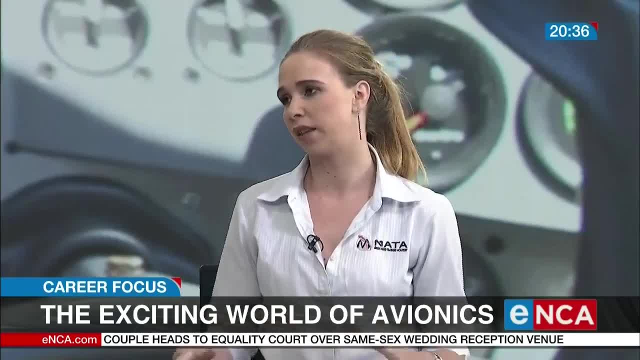 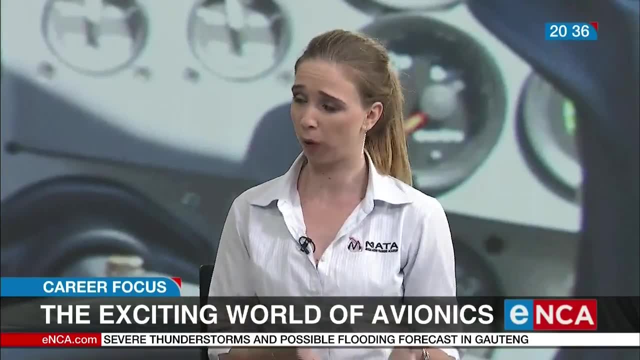 That's the guy that's fixing your instrumentation, Instrumentation, anything inside the aircraft that's got to do with electronics. The work they perform is generally the line on the runway. Aircraft comes in lands, he fixes it and he takes it out. 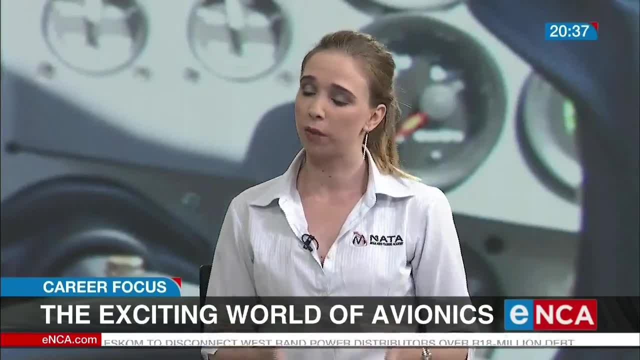 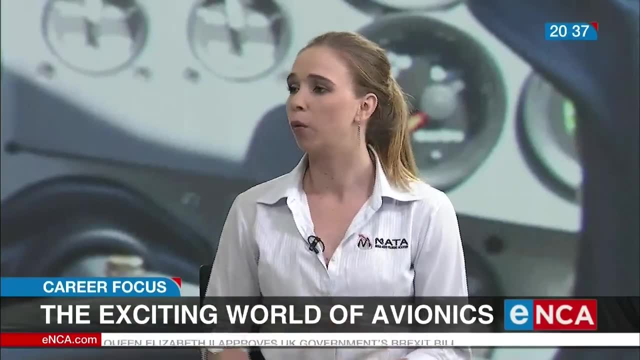 You get another type of avionics engineer, whereas if the instrumentation is not fixable online, it gets sent to a workshop and a category X engineer will then fix it and overhaul it and send it back. Talk us through, then, the academic requirements. 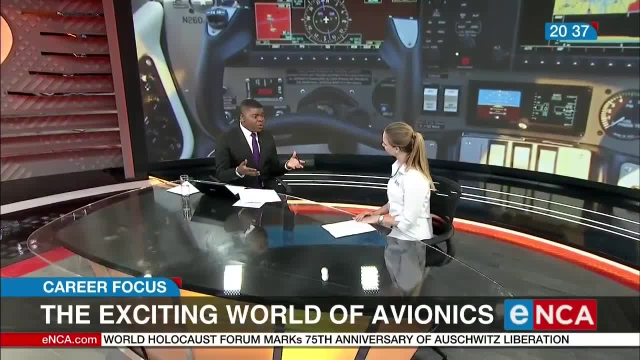 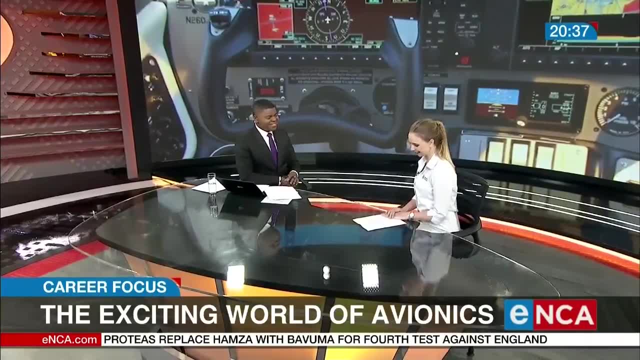 Walking into a university. do I go to any regular university or is there a special school where one can go to take this up? Yes, you can come to our school, for instance. The basic requirements is pure maths and science at a matric level. 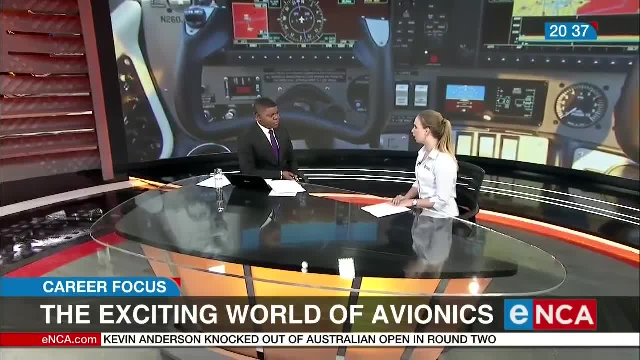 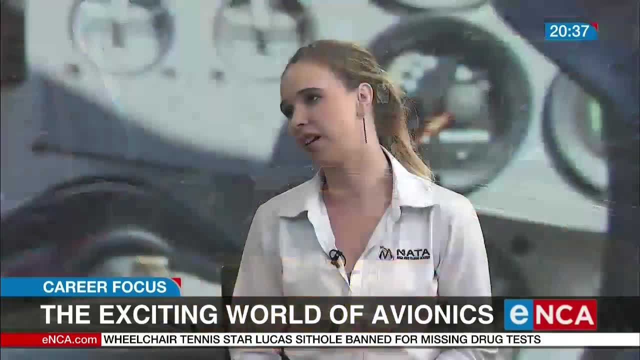 Unfortunately, maths literacy is not acceptable. So that puts me out, then, because I'm a maths person. Well, luckily, you can go do your N3 matric or your maths at any. You can go to any other college that's approved and then you qualify to come and do this with us. 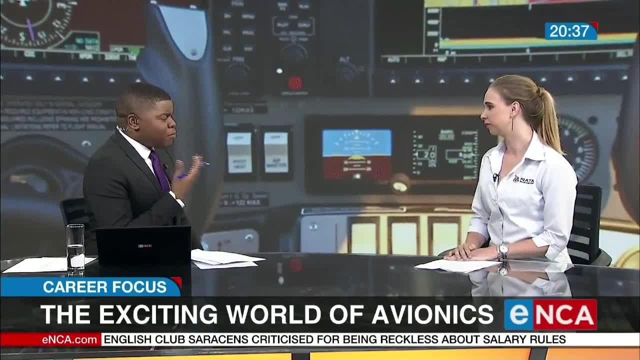 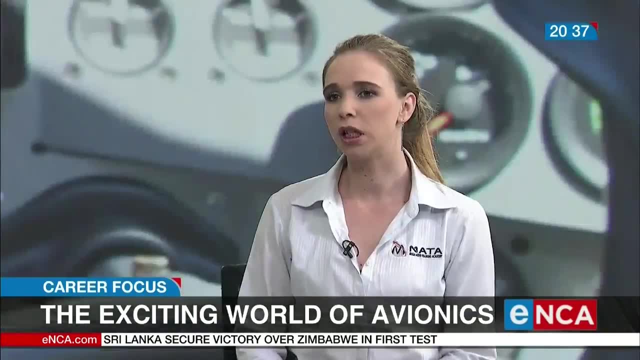 And in terms of the uptake, when you look at the various people who come through, is it still a predominantly male course in the intake? Unfortunately, yes, it is. Luckily, over the last few years we've seen a lot of females come through. 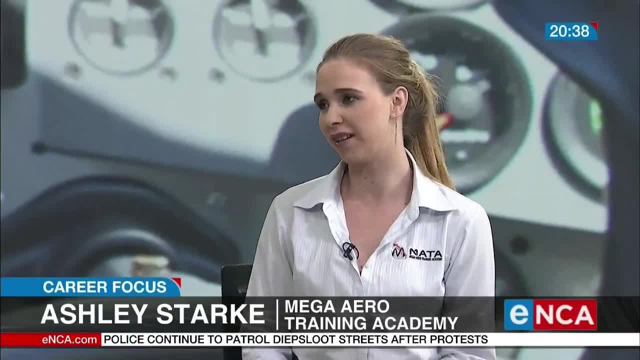 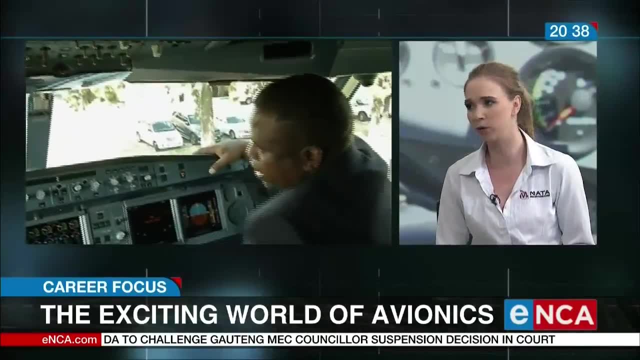 In our institute, our last four or five years our top students has been females. We're vicious, We're vicious, We're vicious. We're no longer accepting the fact that it's a man's world and we're making it ours. 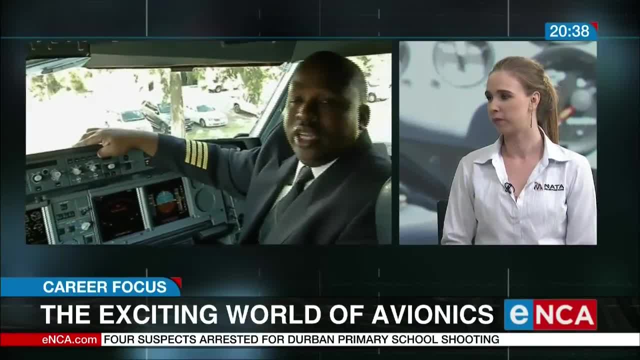 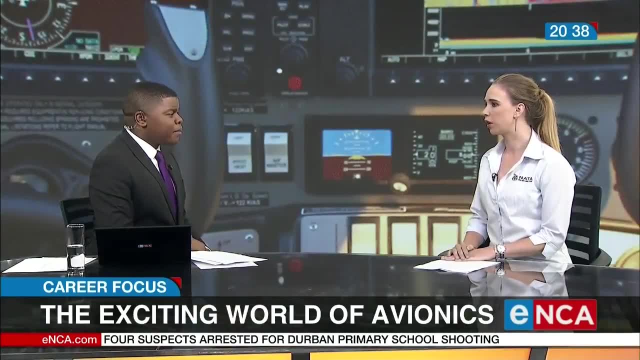 And what about racial transformation? Because, apart from men and women, we also need to see more black people in fields such as this, don't we? Yeah, you know, I don't think in the aviation industry, because it's such a niche industry. 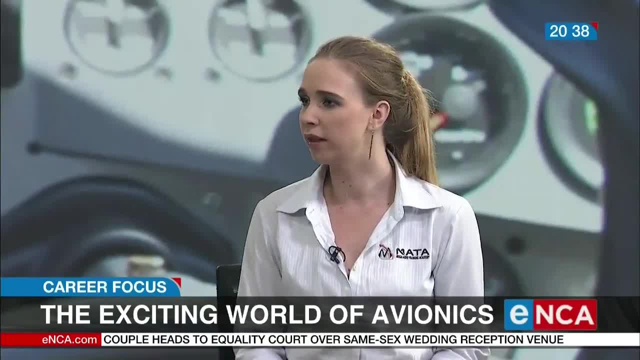 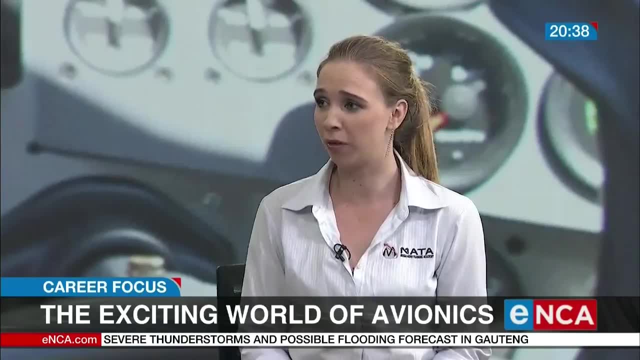 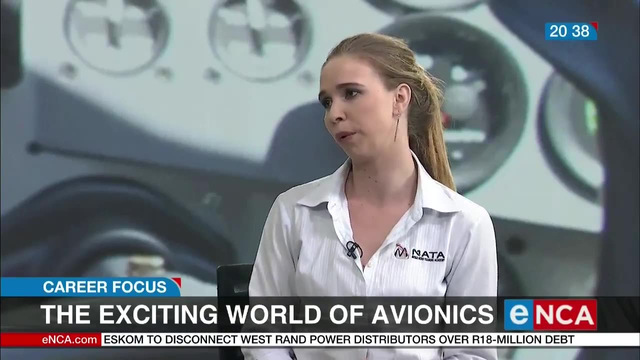 we don't really see that a lot. You know, people are there for a reason and the skills that needs to be applied, the people that go there have a passion for it. Therefore, they work together. They work together really well In aviation. we don't really on the floor under engineers. we don't really have that big racial gap. 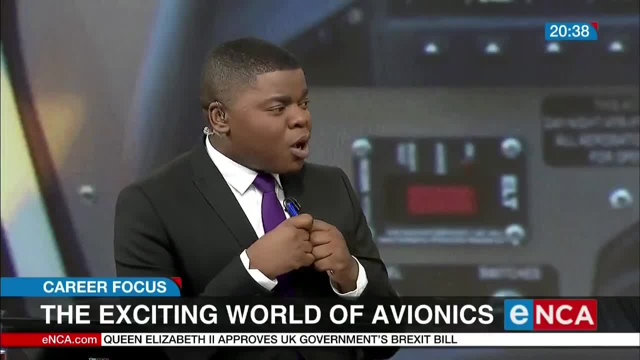 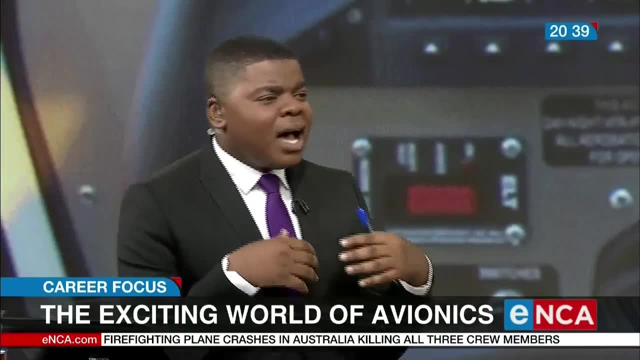 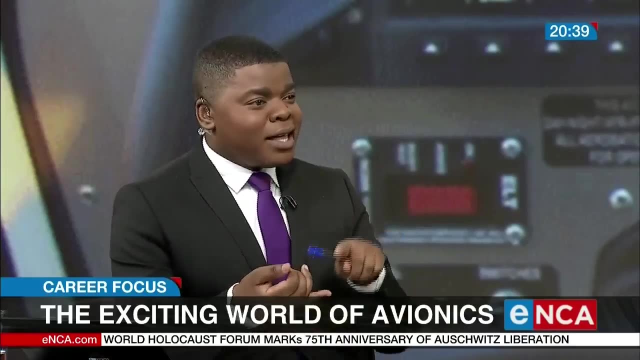 So it's quite a good mix then. But in terms of exposure, I mean, I've not heard about the phrase avionics itself. How much word is out there about these careers? Because when I think of planes, I think of the pilot, I think of the air hostesses. 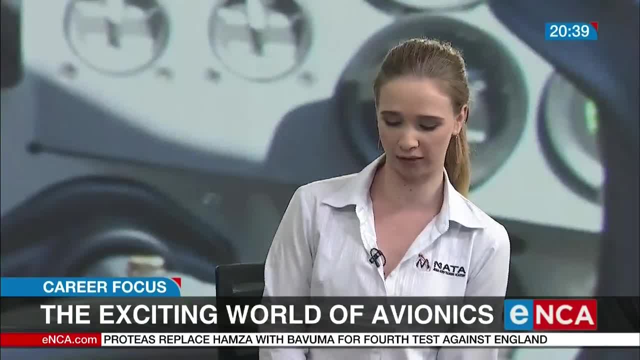 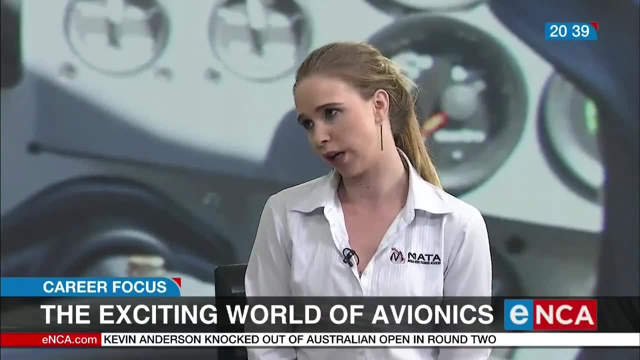 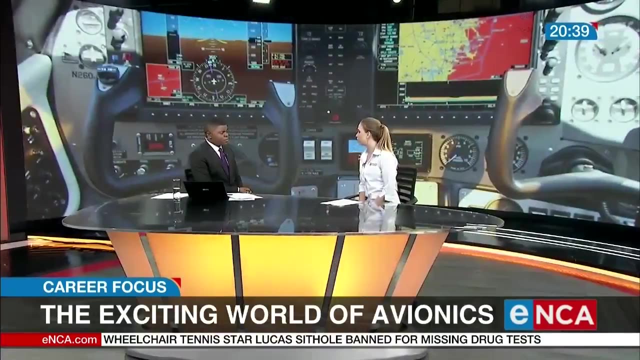 Yes, Look, this is why we are here: Avionics. like I said, it's perceived as a difficult trade because of the academic standard that it's at, which is what we're trying to change. We're trying to encourage the youth to keep their maths and science subjects. 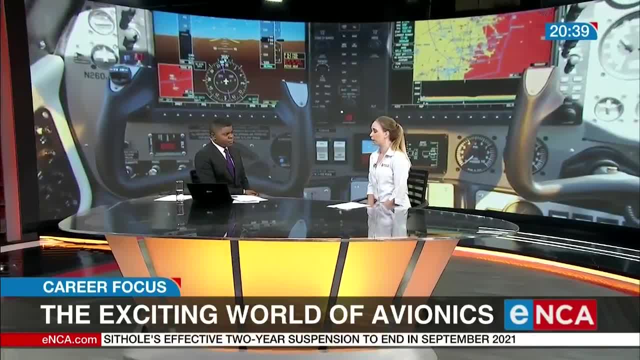 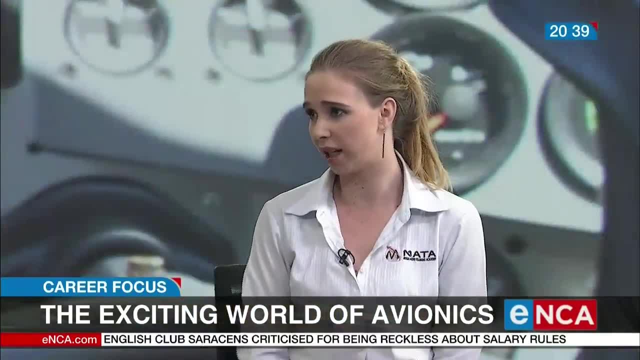 because this will open more opportunities for them. And then you know, we're hoping we're involved with STEM, which is the science, technology and engineering. We're hoping we're involved with STEM, which is the science, technology and engineering organization. 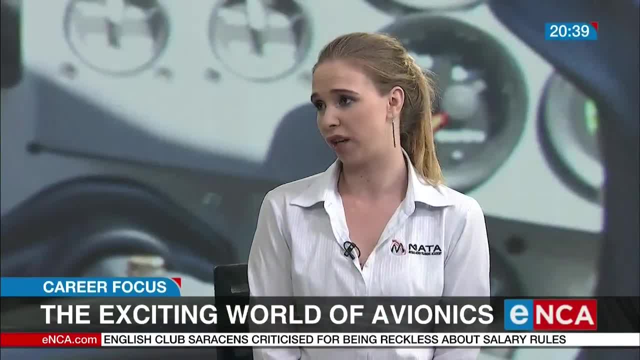 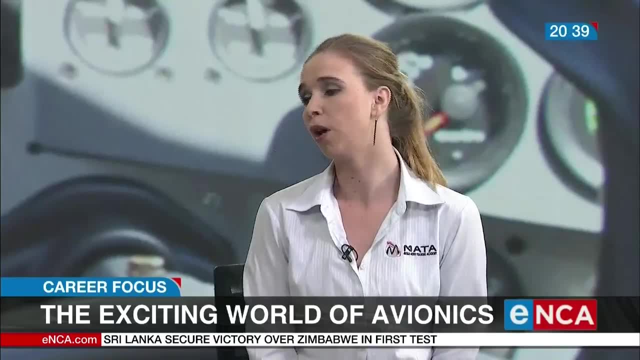 to also encourage the youth to stay, you know, with these subjects and help them and make them aware of the different career opportunities that will become available to them when they stick with us. Given, then, how niche this is, I'd imagine that it's not very difficult. 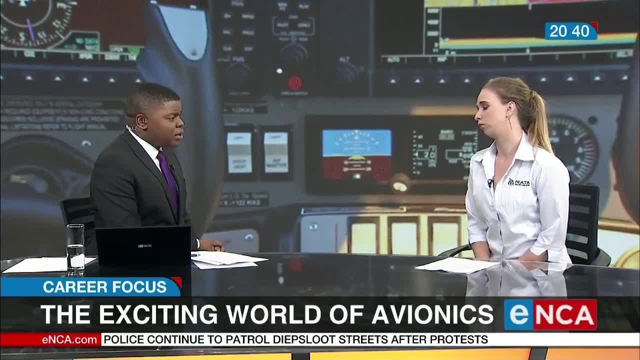 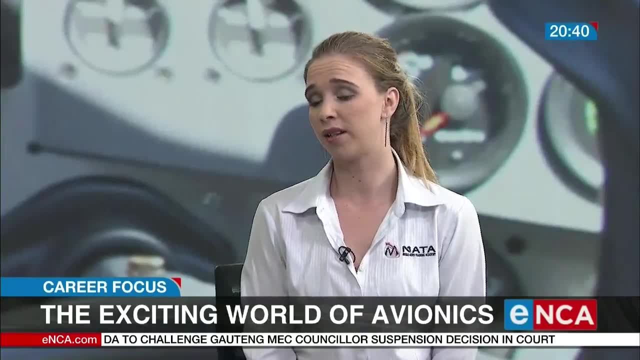 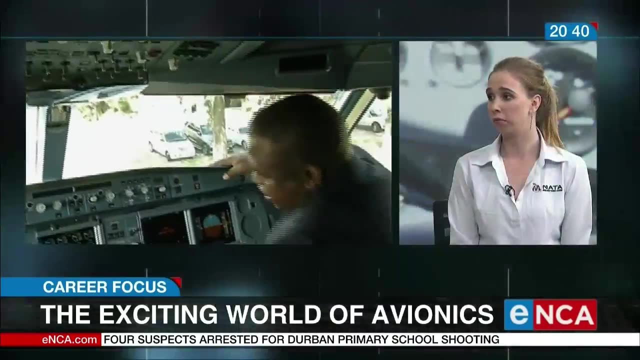 to secure student funding for those people who want to get involved. No, not at all. It's also not cheap. You know it's three years of studying, on-the-job training. unfortunately, you know funding is limited. The CIA has been funding more and more over the years. 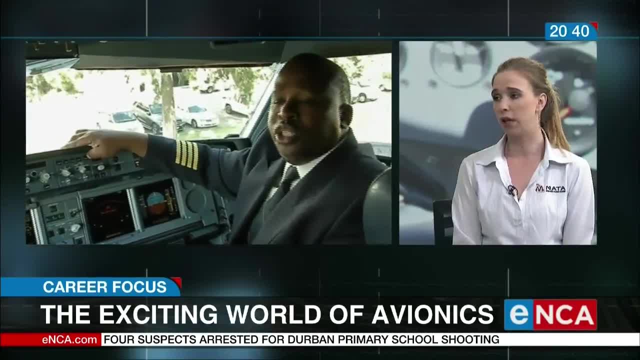 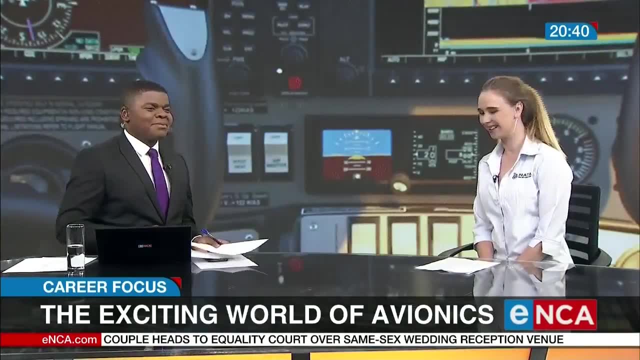 and TITA has been given grants to us, so that's really been great, but it's still not enough. We need more. All right, Ashley Stark. thank you so much for being on Nightline. Sure thanks. All right, that was Ashley, as part of our career focus this week here on Nightline.